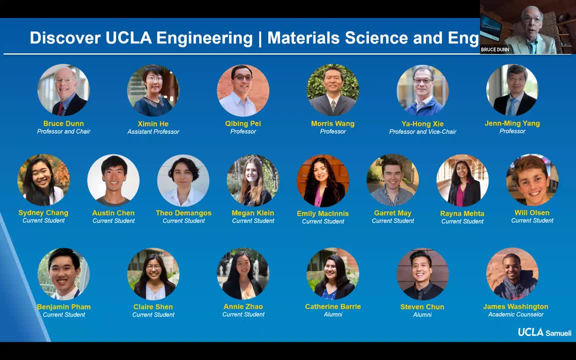 to first of all congratulate all our recruiting people, the people that we're trying to recruit. You have gotten into UCLA. It's exceedingly difficult for people to get into UCLA, and it's even more difficult for people to be admitted to the School of Engineering, So 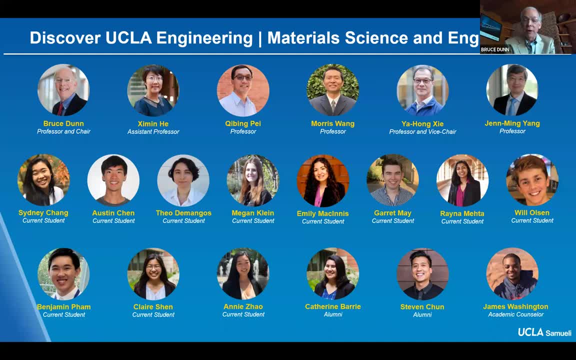 I want to congratulate you really on what's been your outstanding performance in high school, And we all know that prior performance is an indication of future performance, And so we are speaking as a faculty member, but I know I speak for my colleagues. We look forward to having you in our classes so that we can enjoy the things. 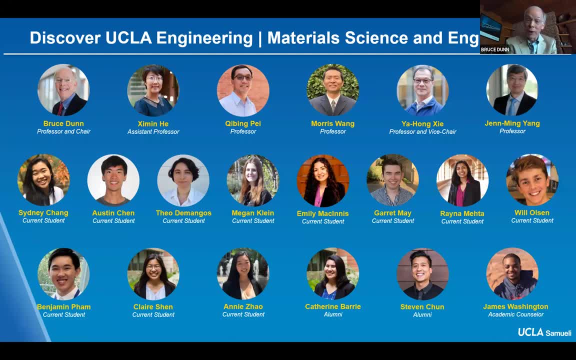 that you bring to the classroom and hopefully you'll enjoy the things that we bring you to the classroom. Okay, so today's program. we have a great mix of faculty students and alumni. The objective is to give you a full idea about what we have here at UCLA in Material Science. 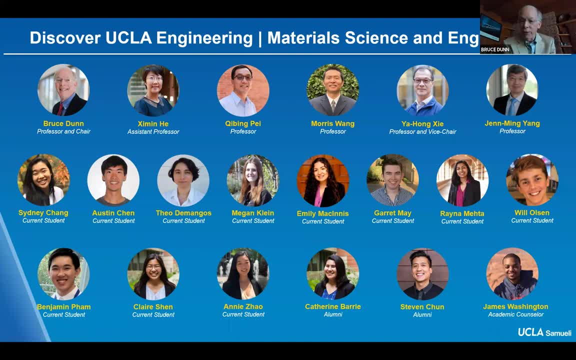 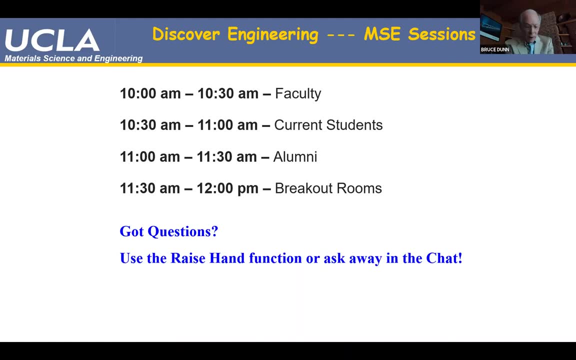 and Engineering, And so with that can I have the first slide. Okay, so this is the rough schedule of what we'll probably keep to, So I want to remind my faculty colleagues: you're given four minutes, So faculty love to talk, but really we've 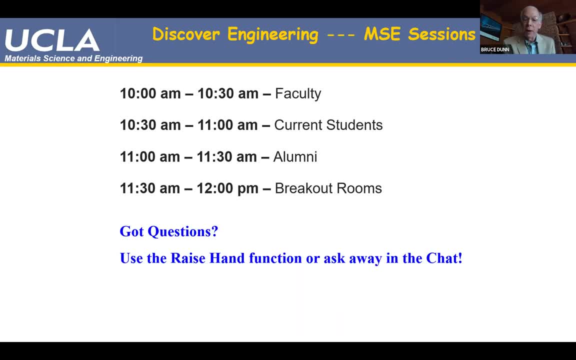 got to keep things on time. So you'll hear from each of the faculty. There might be a little bit of time to ask questions. I think that'll be okay, And then you'll hear from each of the faculty. There might be a little bit of time to ask questions. I think that'll. 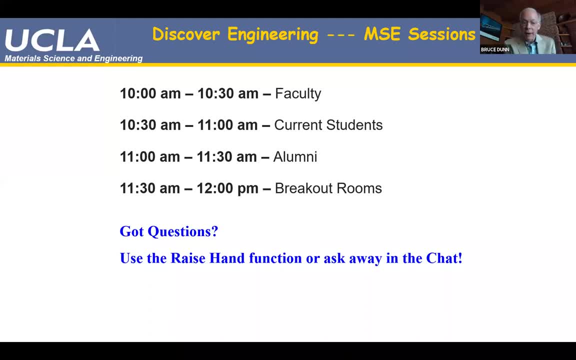 be okay, And then we'll go on to current students, alumni, and then at the end we have breakout rooms. If you have questions as we go, please do not shy away from them. Use the chat, use the raise hand, we'll figure it out. And, Kai, please interrupt us if we. 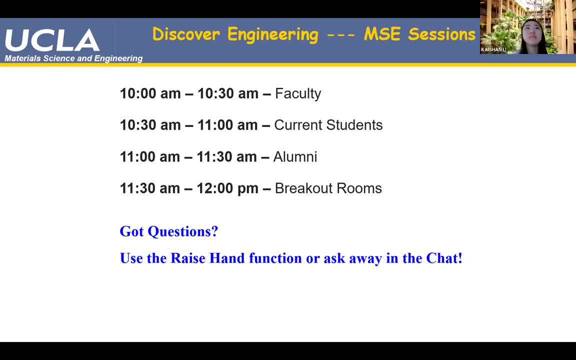 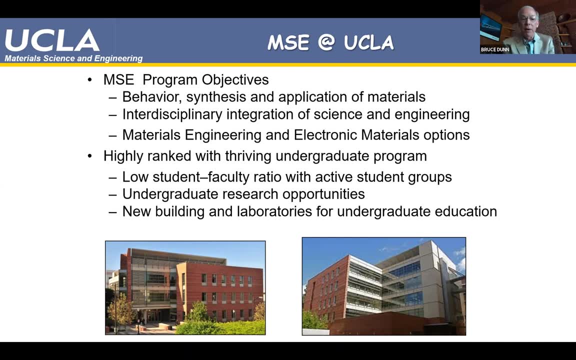 have questions as we go: okay, Sounds good. Okay, all right, So let's get started. Let me tell you a little bit about material science at UCLA, The whole idea here, with material and our material science program we're going to be 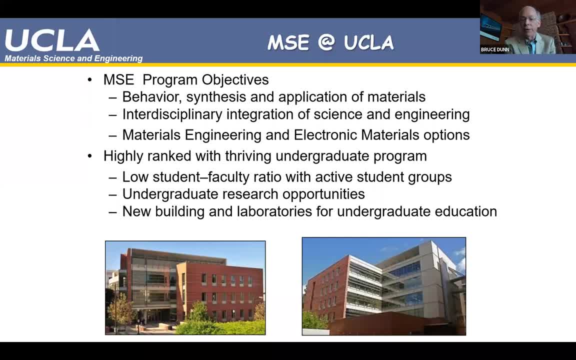 talking about the behavior of materials, also their synthesis, how you make them and how you apply them, And it's very much interdisciplinary because we're combining fundamental science with engineering. All our students are very well acquainted with the other types of engineering because many of the applications of materials are not necessarily 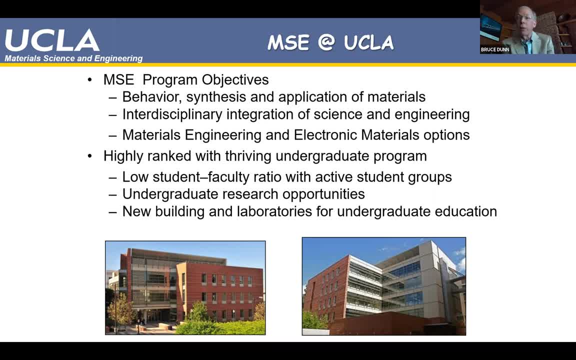 in material science per se, They wind up going into computer science, They wind up going into electrical engineering, mechanical engineering and bioengineering. So there's lots of applications for our materials. Okay, So we're going to be talking about the behavior of materials, also their synthesis. 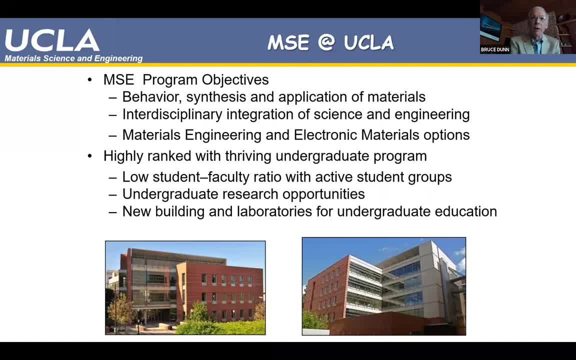 how they form the fundamental basis, And I'm sure you've heard the point that, my goodness, we need a better material, And so that's what we do in material science. That's what you learned about. There's some really great things, I think about the department, The student, faculty. 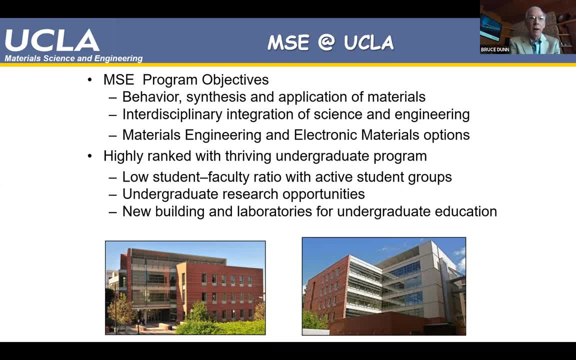 ratio is the lowest in the school, which means we have more faculty per student and that there's great research opportunities. I'll talk a little bit about that. And we moved into a building. it's now about seven years old but it's still quite new And, as 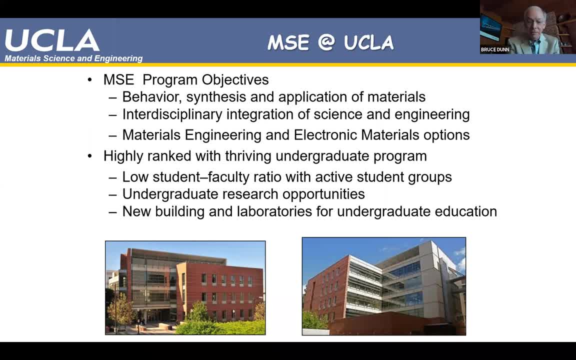 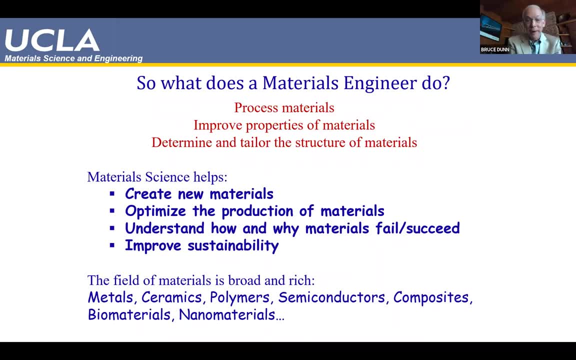 you can see it's not as old as campus buildings. go Next slide. Okay, So what does a materials engineer do? Well, that's the whole idea that we train you to be a materials engineer. You learn about the processing of materials. How do? 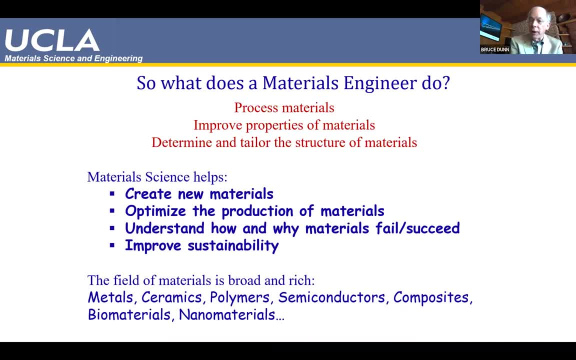 you make materials into useful forms? How do you create new materials? In that sense, part of material science is extremely creative because of the fact we are doing things that nobody's done before, And so this is really why we are. you know, we're doing a lot of. 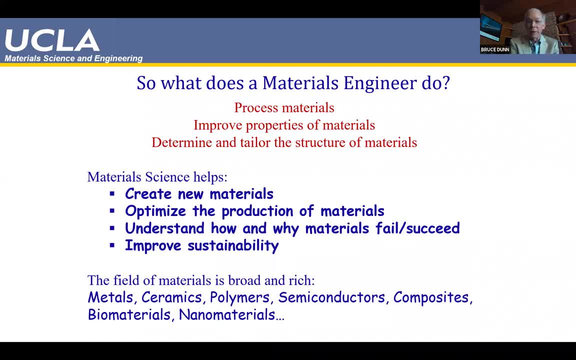 research. We are very excited about this discipline because of our opportunities to help in so many different areas of society. really, Production of materials is extremely important- You learn about that as well- And also very important. why do materials fail? because lots of times, you learn a lot when something doesn't work. 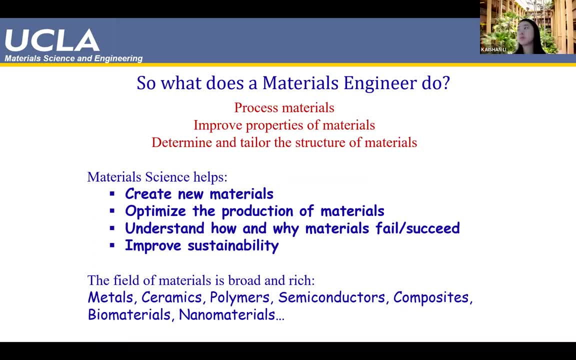 So there's a number of different materials that we focus on. There's metals- that's the traditional background in materials science. There's ceramics, polymers, semiconductors, composites, biomaterials, nanomaterials- All of that. all of that is within our umbrella. 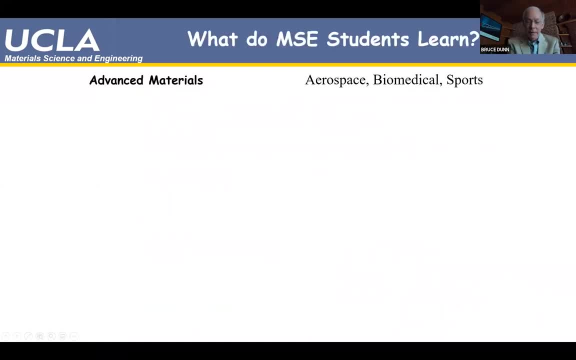 and all of that you learn about Next slide. So let me just give you a very, very quick sort of overview of the kinds of things we talk about, If you could hit the next button. Okay, So advanced materials. that goes into. 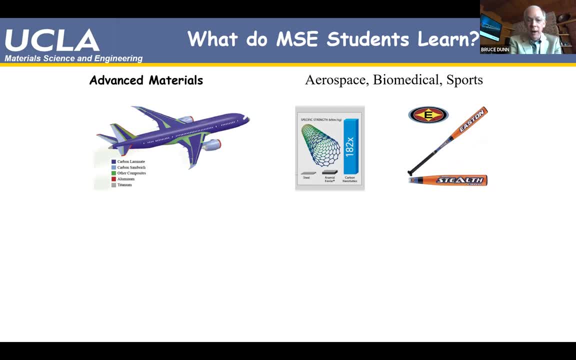 aerospace, without question, And one of our faculty Professor, Jemim Yang, is here. He'll talk a little bit more about that. We also do a lot of work related to biomedical materials, and sports, of course, have a lot of characteristics in common with both biomedical materials and 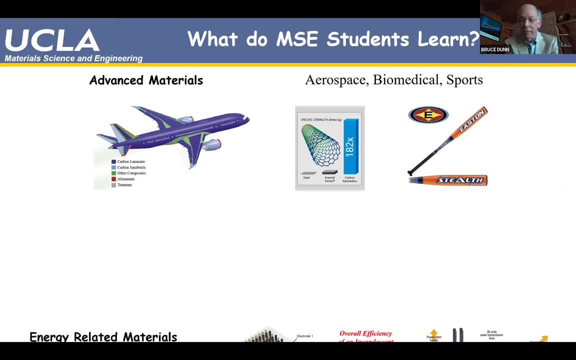 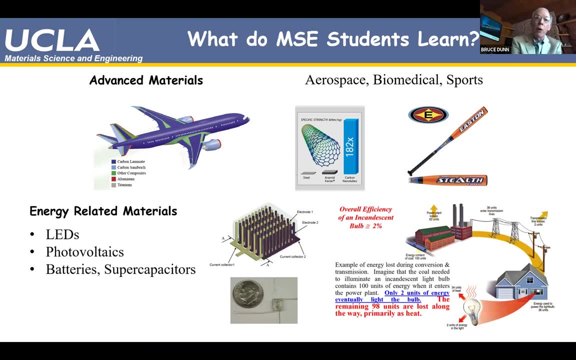 advanced materials, especially aerospace materials. Next button: Great. And then, of course, energy today is extremely important. We have a very active research program and also you learn about in classes A lot of materials that are used for generating power, such as photovoltaics. 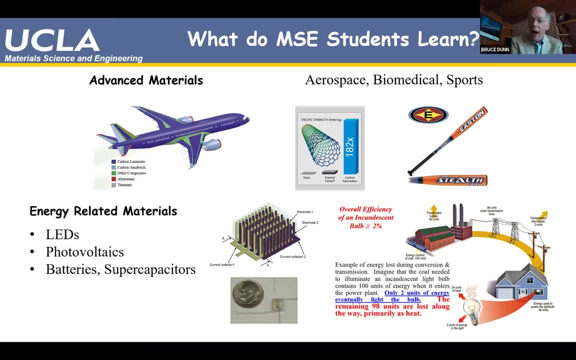 other materials that are used in storing energy and generally how this all works together so that we are able to store energy that comes in from sunlight, for example, and use it in homes. And so this is, you know, sort of the whole idea behind sustainability And 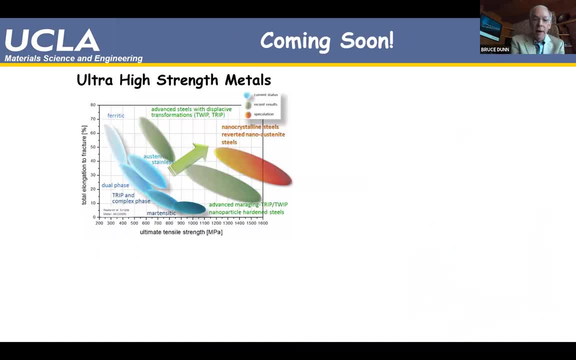 those principles are also taught. Next slide: There's a future, and this is really the things that go on in our laboratories. We are working on ultra high strength materials. A lot of these are nanomaterials. There's a lot of materials that are extremely strong, And this is very exciting, Of course. 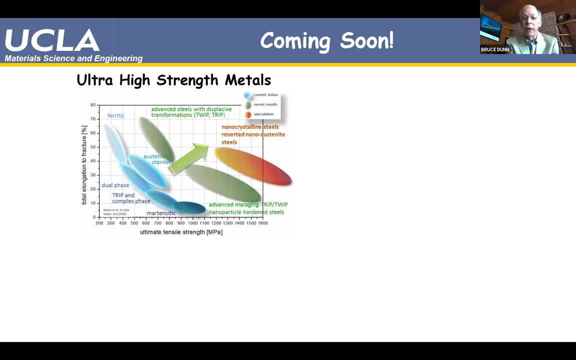 it's all at a research level, but this is the kind of thing you can look forward to- The next slide. And then there's all sorts of smart clothing: the idea that you're going to be wearing things that are going to be telling. have all sorts of sensors on it to 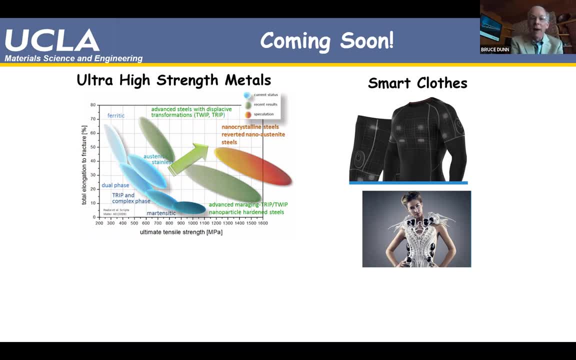 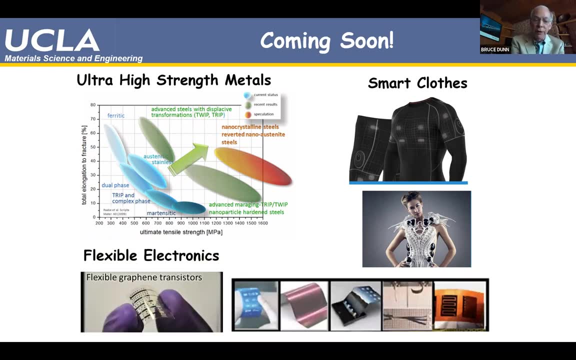 tell you what you're doing, generating power at the same time And what, and just having complete flexibility in what you do. And then the next slide is sort of the enabling feature behind the smart clothes, And that's the whole idea behind flexible electronics. 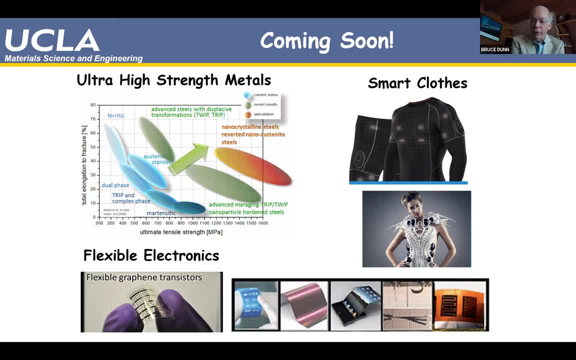 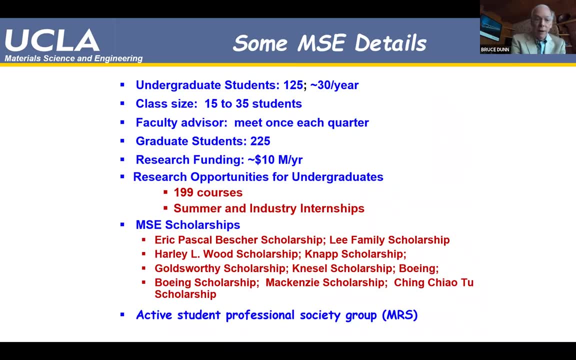 no longer with things just beyond rigid chips there are going to be on all sorts of different backgrounds and so forth, So you can bend them and they can flex them and so forth. So that's the future, some of our details and our department. the total number of students. 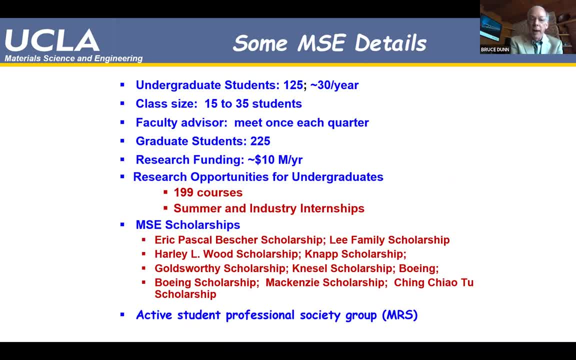 we usually get about 30 per year, which is great, Um and so. the class size is always less than seven foot. each and a half feet of cetos that we integrated to our leading temperatures. Feedback logoum: I'm not going to, I'm going to show. 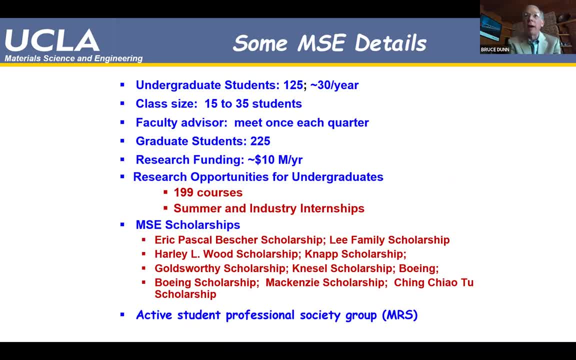 you some slides of the of each of the of the methods are, and that I'm not going to cover the than 35, and that turns out to be really important, certainly from the standpoint of student-faculty ratio and accessibility that we have. We have a very large graduate program and that just has 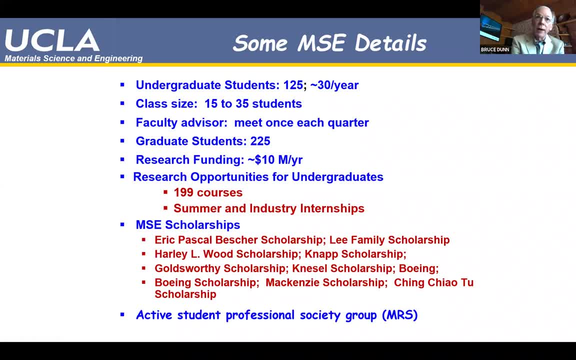 to do with the nature of material science. A lot of people go into material science in the graduate program because of their backgrounds in chemistry or physics or even biology and certainly some of the other engineering. We have a very active research program- $10 million per year, puts us. 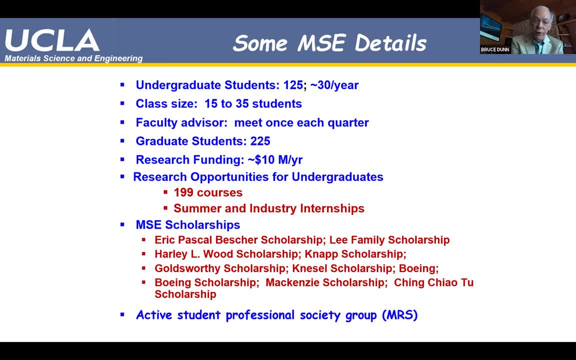 about the third most department in the School of Engineering, even though we are the smallest department. So there you can figure out that we are very active in research, Lots of opportunities for undergraduates to get involved in research, and we actively do that through courses as well. 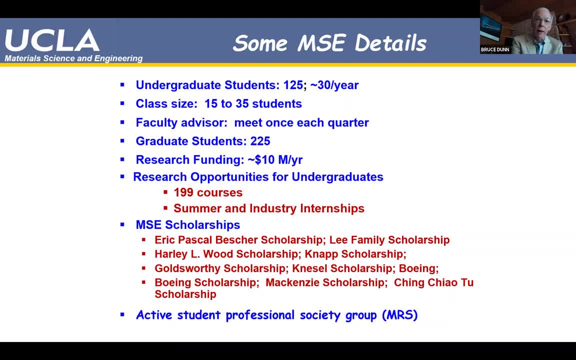 as just students just being around and helping out in laboratories. And, of course, there's a very active program by our MRS organization that helps students in terms of their internships, And then, finally, there's the aspects of a number of different scholarships And, again, because we have a low number of students, these things are 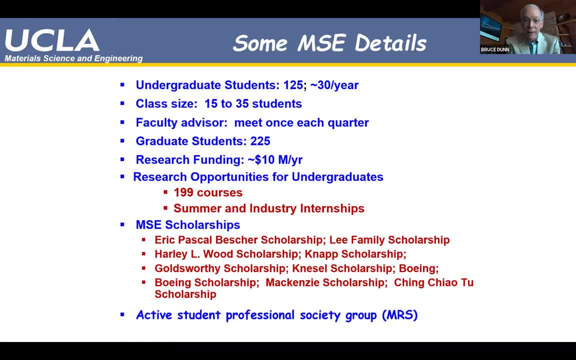 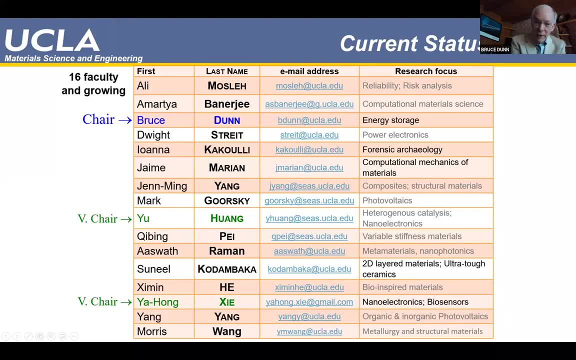 reasonably well distributed among our students. So I think that's my last slide, Is that right? Oh, here's just a list of faculty, And the last thing that I just want to mention is that we are currently 16 faculty and we're growing. We've added three faculty in the last 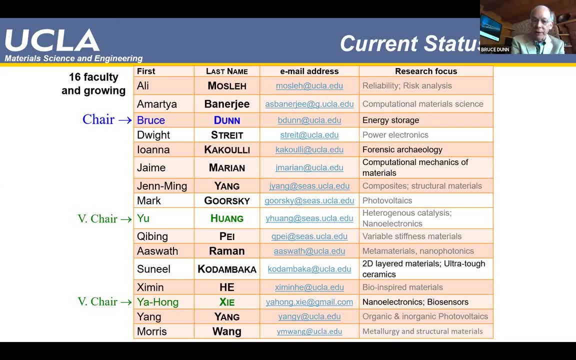 three years and we anticipate that we're going to continue to add faculty over the next several years. And the reason is because we're going to continue to add faculty over the next several years. And the reason is because we're going to continue to add faculty over the next several. 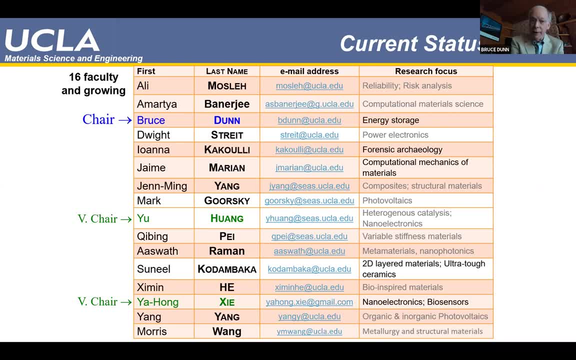 years, And the reason is because we're going to continue to add faculty over the next several years And the way that you keep up with these changes are by adding faculty who have these new talents, these new skills, which certainly drift down very rapidly to the classroom. 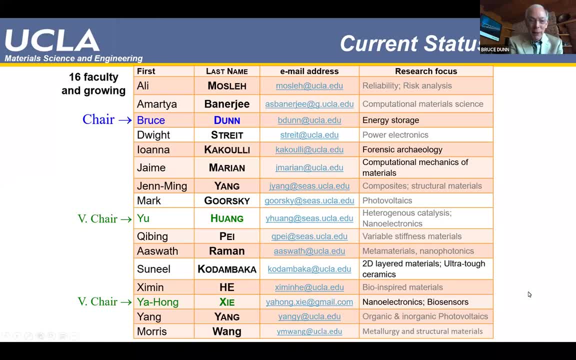 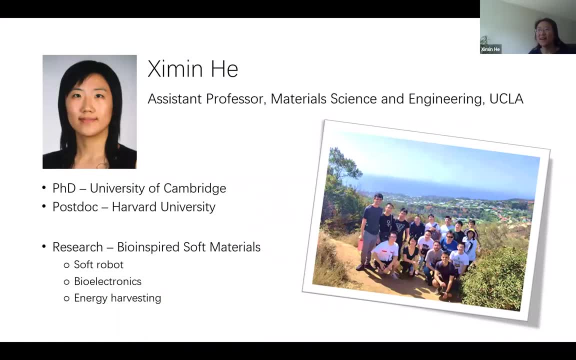 Now I think I'm finished. I think that's my last slide And with that I'm going to introduce Professor Hie. So Ximin XIMIN HIE. Yes, thank you Bruce. Hi everyone, I'm Ximin Hie. I'm assistant professor in this. 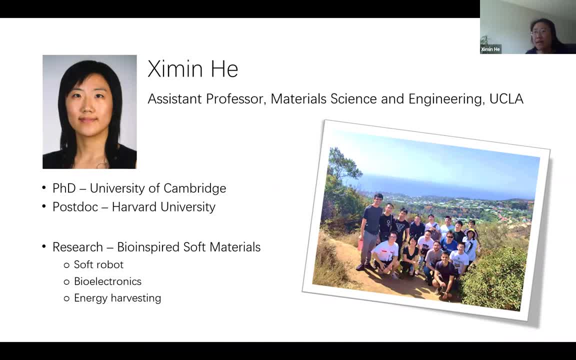 department. Before I joined USLA, I did my PhD in chemistry in the department and I did my PhD in University of Cambridge in England and then went to Harvard University for postdoc. So my research is bio-inspired soft materials, So basically we're focused on different kinds of polymer. 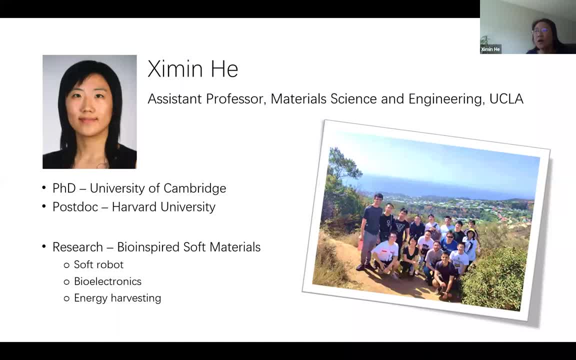 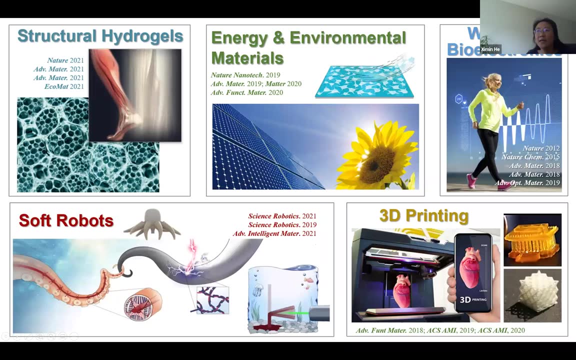 polymeric materials for applications in soft robot bioelectronics and energy harvesting. So in next slide you're going to see if, Kai, you can click Yes. so basically, we study different kind of polymers. So hydrogel is a type of polymer that is very close to our tissue. As you can see, it has pores and it's very soft. 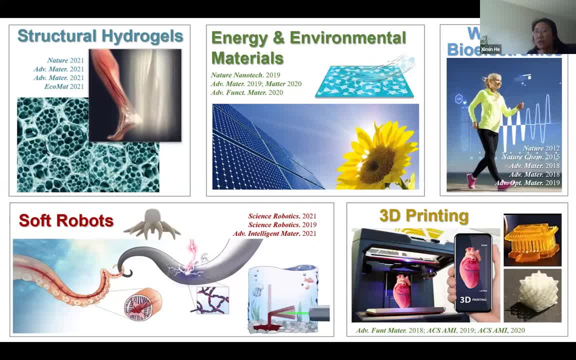 contains water, but people usually want to use it with the like high robustness. Therefore, we study how we can tailor the nano microstructure to make it approaching the bio-tissue that we have in our body, and you probably cannot imagine. with this kind of a soft, gooey material we can actually do many other things, For example: 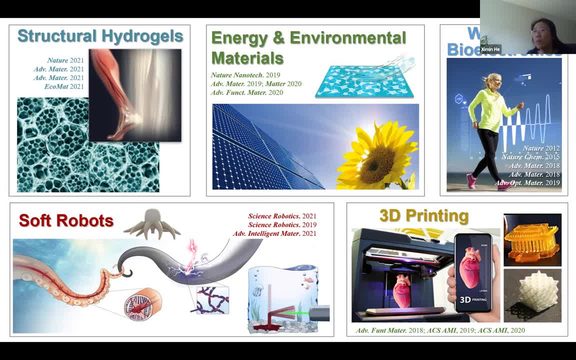 we can utilize it to create like anti-icing coating, or use it to mimic the sunflower to track the sunlight across the sky, and we can make it like a wearable electronic materials to monitor our bodily function. We can also make it like a smart material to mimic the muscle. 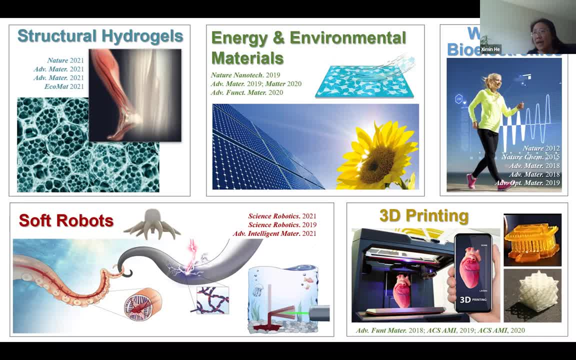 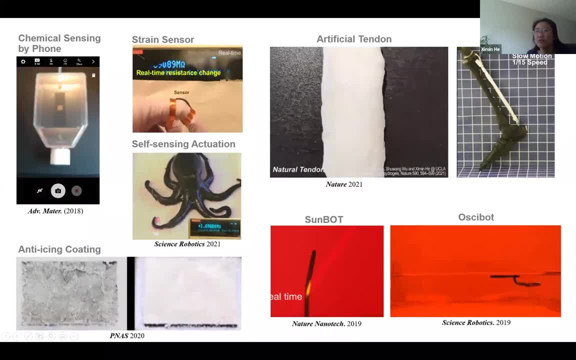 and we can also 3D print it into a compact structure. In the next slide, Yip Kai, you can help. In the next slide you will see a bunch of videos to give you a rough idea and how we can utilize to sense the chemical molecules. 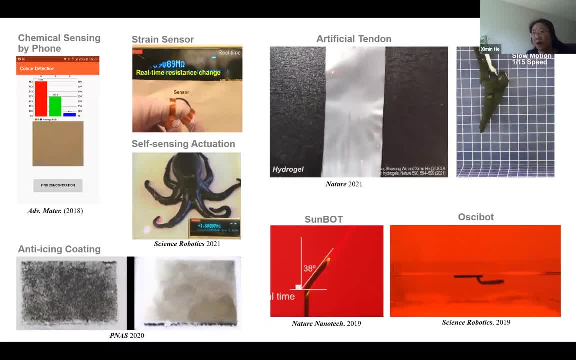 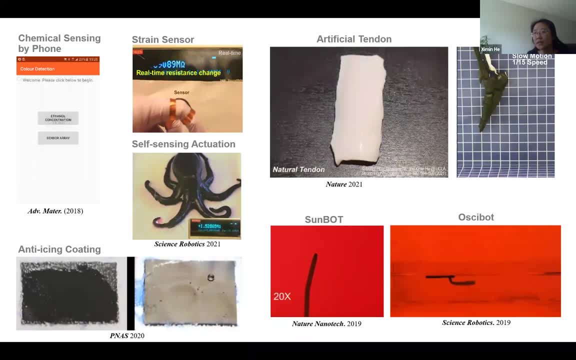 or we can use it to like a band-aid on our finger or body to measure the real-time movement, or we can use it to track the light, as you can see in the sunbot, or we can make it like a self-propeller to swim in water. 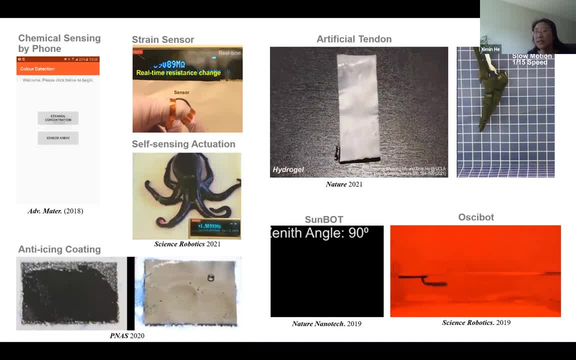 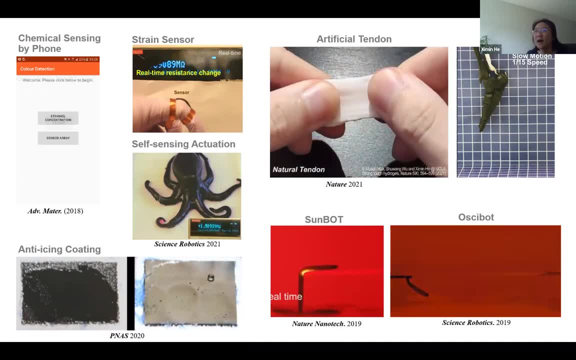 and also we can chemically functionalize it to make it anti-icing, so that the surface won't have an ice cover. So I will just end here because I only have four minutes. but it just shows how diverse materials can do, even with the soft materials. 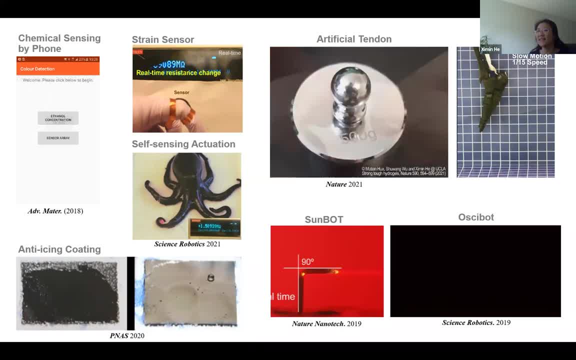 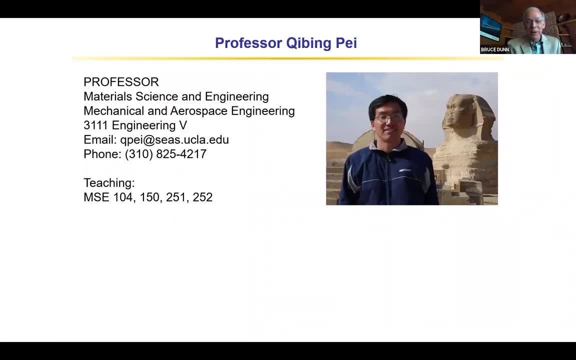 And later you're gonna see many other type of materials from our other colleagues. All right, thank you. Great. Thank you, Ximing. Okay, Ximing, all yours, Thank you. Maybe he lost power, like he warned us. Yeah, let me say that, Professor Pei. 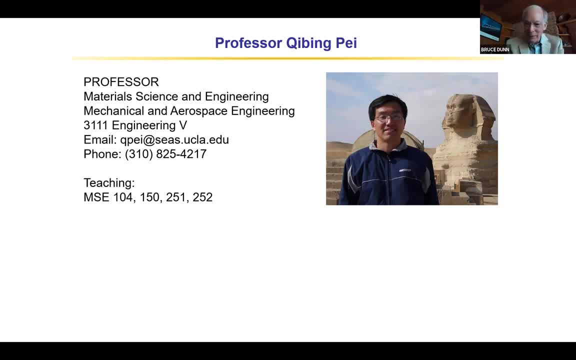 was having a power outage at his home today, he said: And so he didn't know how bad it was going to be. I think we're gonna have to move on rather than wait the two hours for his power outage to stop. Okay, so that's okay great. 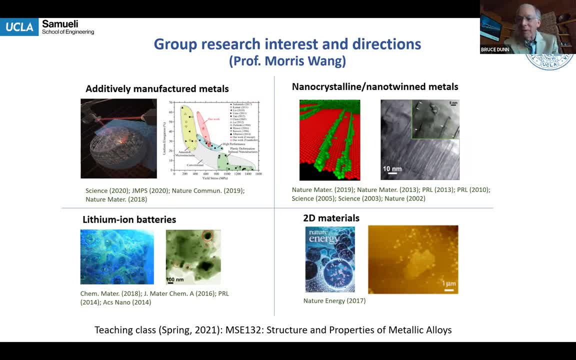 And then Professor Morris Wang, our newest addition to the department. Thanks, Bruce, I'm here. Hopefully my house also says power outage, but I have power right now. As Bruce said, I'm the newest member of the department. I just joined the department three months ago. 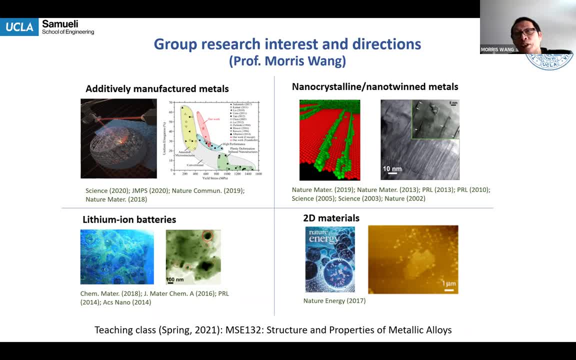 My group is mostly working on ultra-high-strength materials, but we're having a lot of fun. essentially, Most of my group's work is kind of summarized here. One of the most important areas is 3D printing or element manufacturing, And its broad concept is different type. 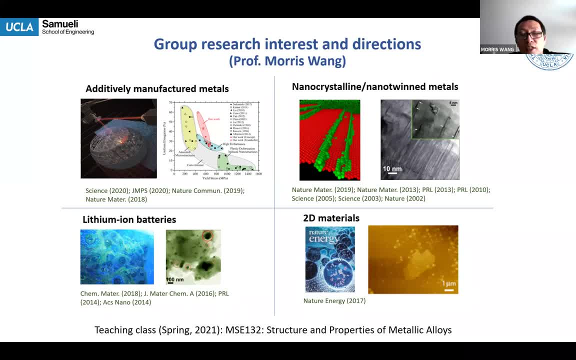 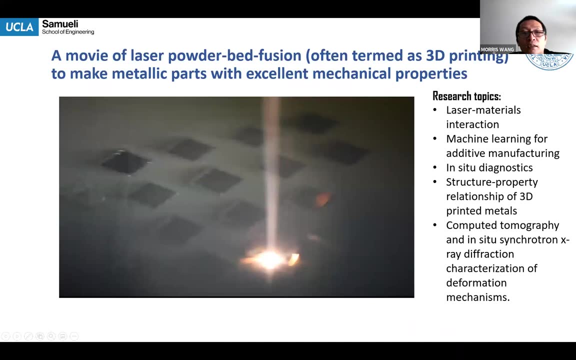 of element manufacturing approaches, And then we also try to use that approach for the nanostructure material as well as some of the battery applications for the energy storage. Next slide, please And sorry, And the type of element manufacturing we're most interested in. 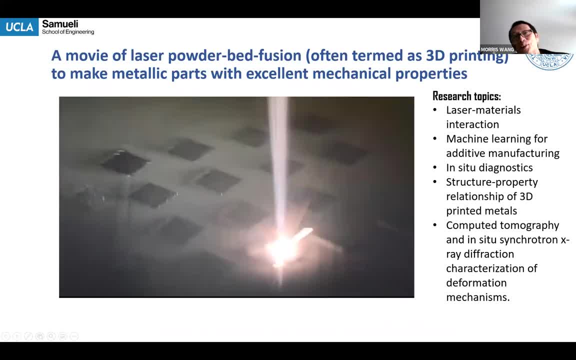 this is actually a movie, I don't know. Oh, it's playing great. Thank you, Yeah, the approach we're using mostly using approach so-called laser powder fusion. Basically it's laser using laser to make powders. 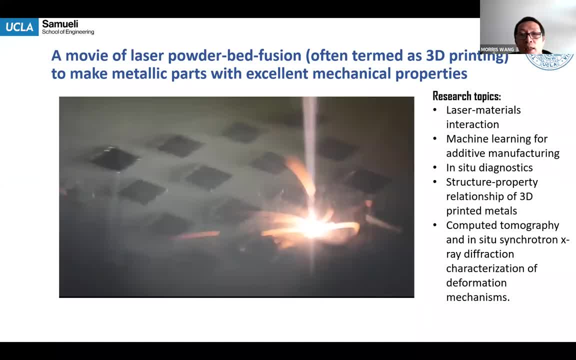 and making materials with good mechanic properties, And so the research focus area is basically, we mainly use laser. We try to understand how the laser materials into action and, using machine learning- because this is very complex processes- try to identify what kind of microstructure we can make. 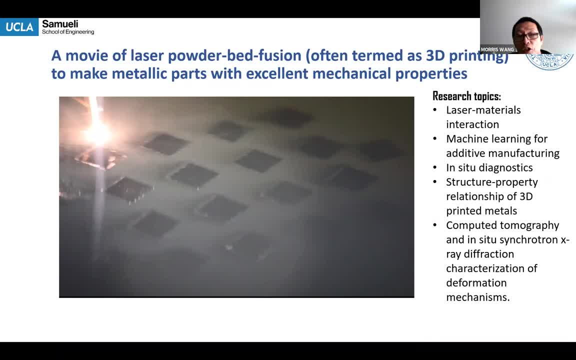 And then we mainly focus on, obviously, on this so-called structural problem relationship, And then we're using a lot of state of art calculations in the group, including computer tomography, in situ, X-ray diffraction, try to understand the materials behaviors. So we are very eager to you know. 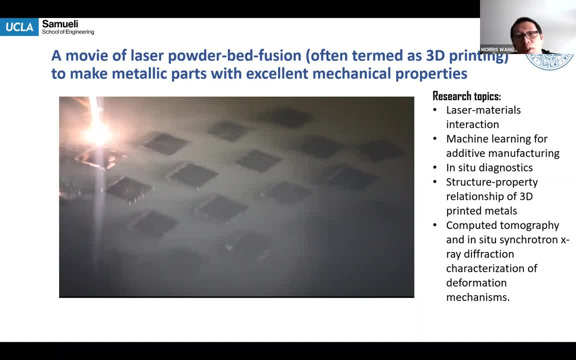 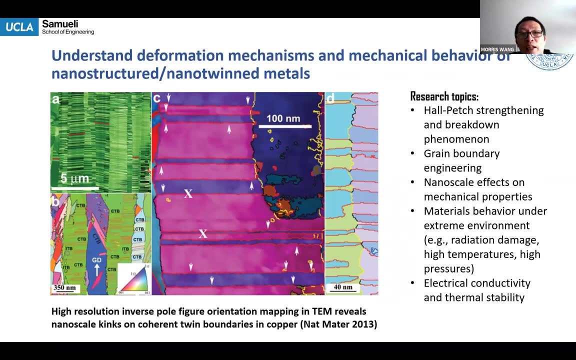 recruiting undergraduate students as well as graduate students. working on, you know, this fun project, this 3D printing For us, we consider the material synthesis tool, making new materials. basically, Next slide, please. So the, as Bruce also mentioned. 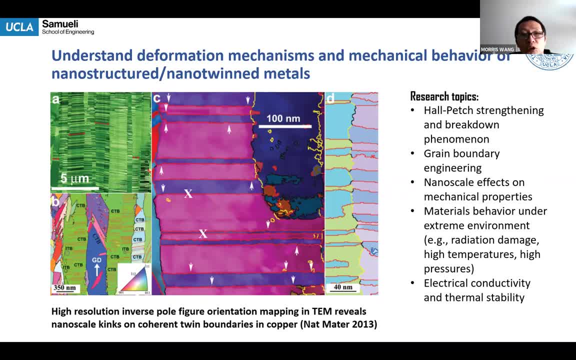 one of the- you know, our strength department, and also my group, is working on so-called ultra-high stress materials by trying to understanding how the materials can reach the limit, And one of the scaling you know we call this called Hoy-Patrick scaling. 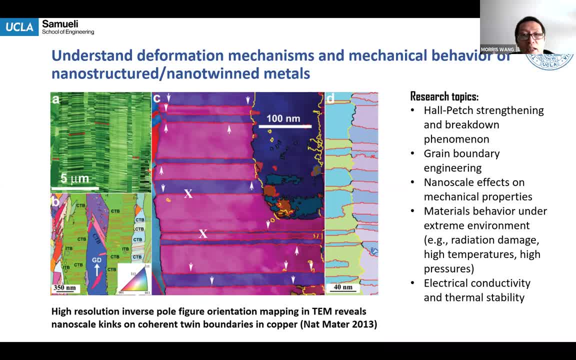 Essentially the scaling, eventually, you know, from the fixed, this perspective is going to break down And we try to understanding, you know, how these materials behaviors, how we can reach the max strength And two type of materials that we started quite a bit is. 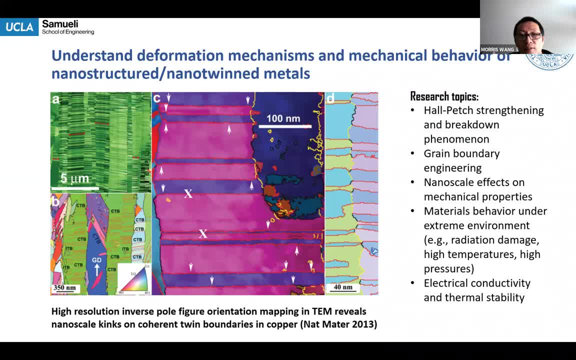 one type is called a nanocrystalline materials with a green size less than a hundred nanometers, And the other type of materials, so-called nanotwin materials, is relatively new. which materials actually is strengthening this figure showing there? 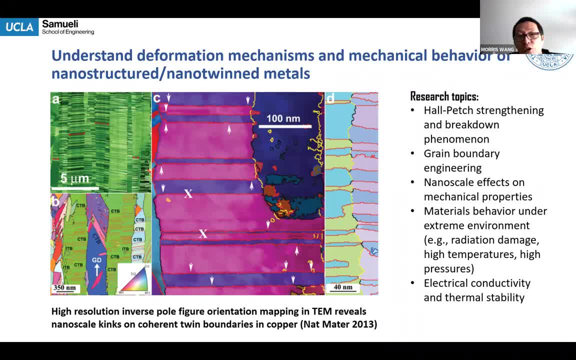 Materials actually is strengthening by so-called nanotwins. It has advantages because nanotwins actually doesn't scatter electrons as much as high angle green boundaries. Therefore it's giving you understanding. electric conductivity is worth high strength. Next slide, please. So this is my last slide. 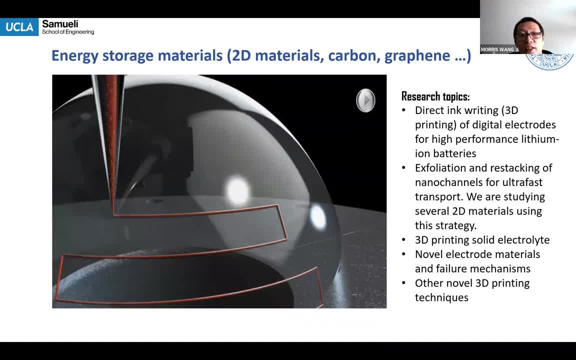 This is actually working together with Professor Wu-Stang and on the energy sorority, So we are thinking about using 3D printing. In this case is what we call direct ink writing- very interesting material approach. It looks like you know. 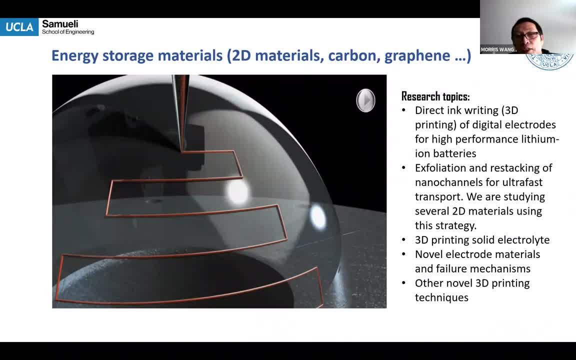 oversimplified but in reality can be very complex. The idea is we're using so-called direct ink writing to make a 3D electrode, digital electrode for the leasing iron batteries or supercapacitive performance, And this is also very fun And we are also looking, you know. 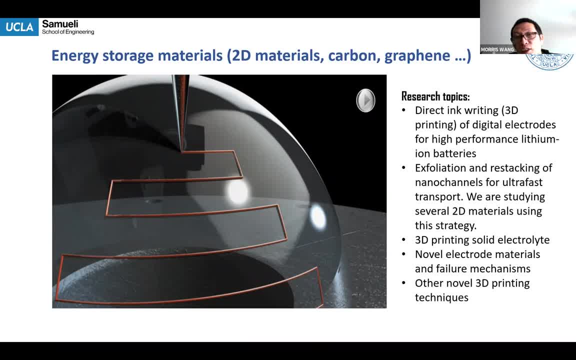 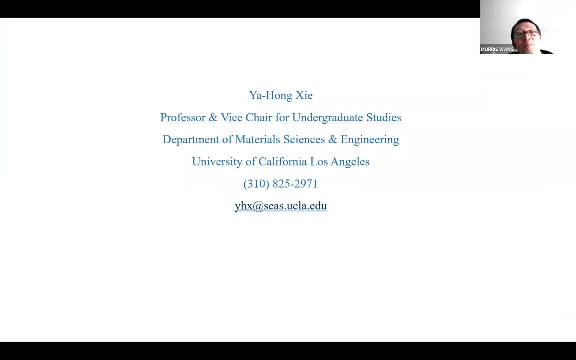 for undergraduate, if it was a master student group, to join the team. Thanks, So that's all I have. Great Thank you. And next will be Yu-Hong Hsieh, who's the vice chair for the department, Yu-Hong. 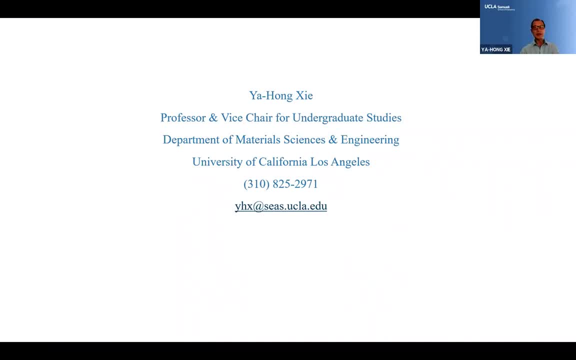 Okay, So it's my turn. Hello everyone, Welcome to UCLA. I have been. my name is Yu-Hong Hsieh. I've been with the department for over 20 years. I'll think back that time really flies Prior to that, actually. 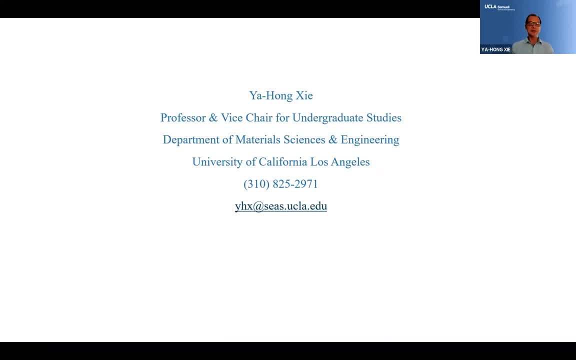 even when I joined the department, I was a mid-career, So I actually worked in a company for 14 years before joining the department, So I've been around Now. incidentally, Professor Bruce Dunn, when I was doing my PhD at UCLA in electrical engineering, 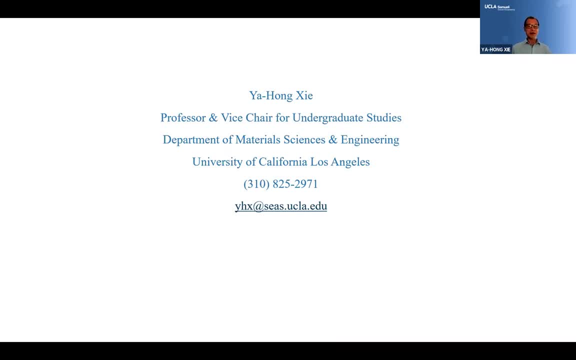 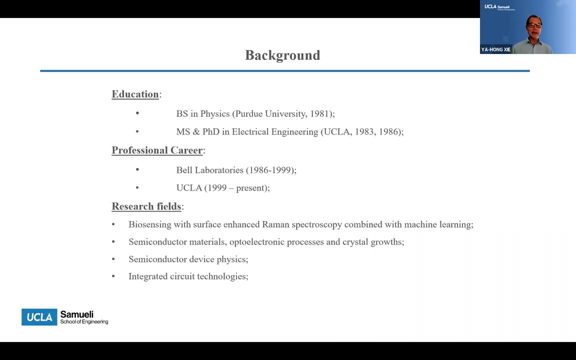 Professor Dunn was my professor in one of the courses till today. Actually, I teach that course. So you know there's quite a bit of history tracing back. So Kai, next slide, please. Okay, Here is a brief history of my professional background. 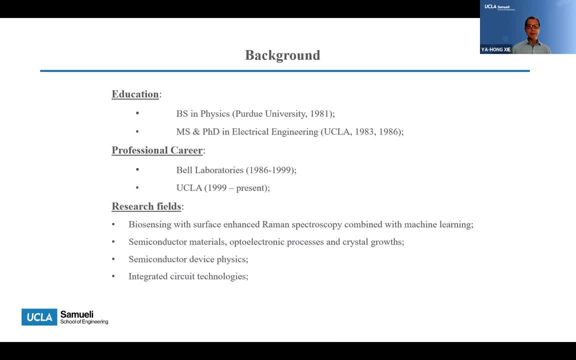 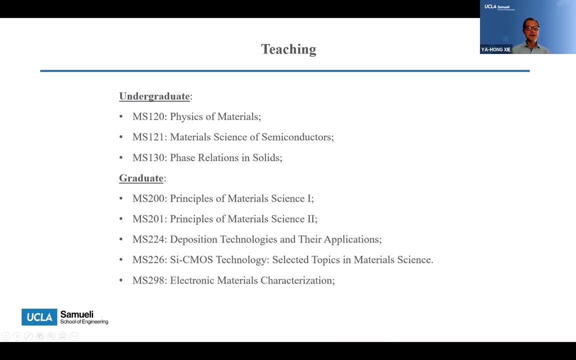 and my research area have to do with biosensing and also semiconductor materials and devices. Next slide, please. And also, you know, I am the first generation immigrant. I guess, as you can see, Came from China, As quite some of you, I think. 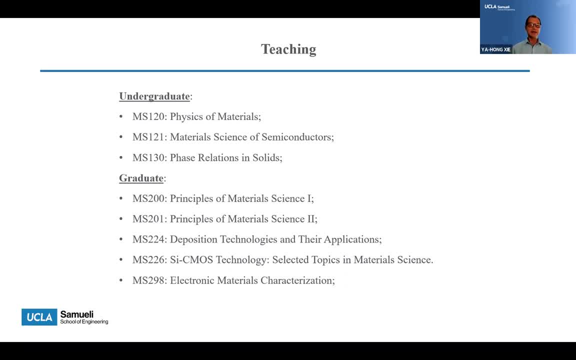 participating in today's meeting might be also have that similar background. Okay, As far as my teaching is concerned, I, you know, teach three undergraduate courses and four or five graduate level courses, And I will see you when you get to your third year. 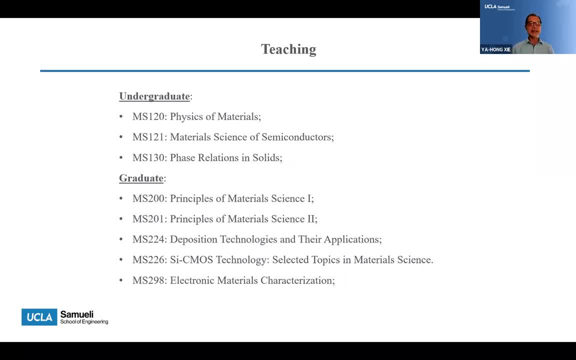 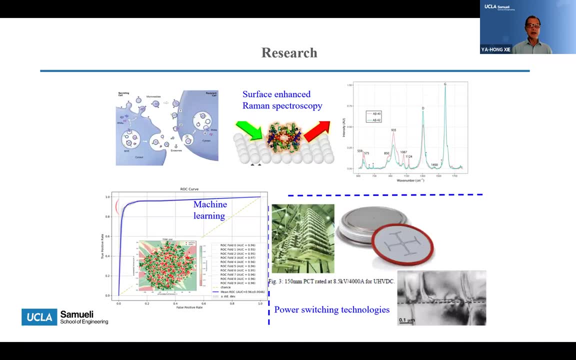 fourth year you'll have to take some of these courses. Next slide, please. Next slide, please. Okay. So a few words about my research On that front I would like to share with you because my educational background is truly non-material science. 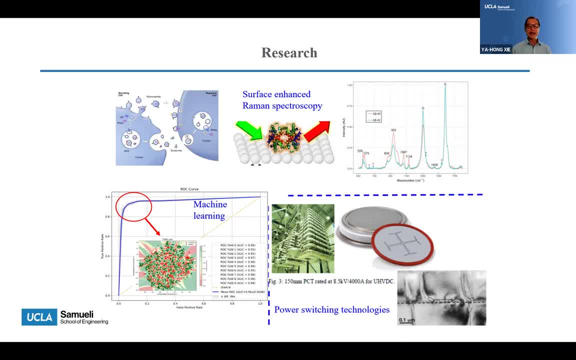 It's actually physics for my undergraduate degree and electrical engineering for my PhD, master's and PhD, So I might be able to provide a short talk about my research. So I'm going to start with a sort of a slightly different perspective as to what is material science. 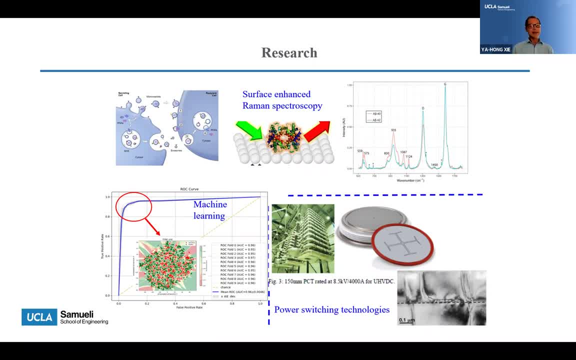 To me, actually, material science is the science that we study how, by adjusting the composition and the structure of materials, to expect certain kind of a response of a particular material under the influence of external stimulation. right, What kind of external stimulation? Well, if you press the material, that's the structural property. 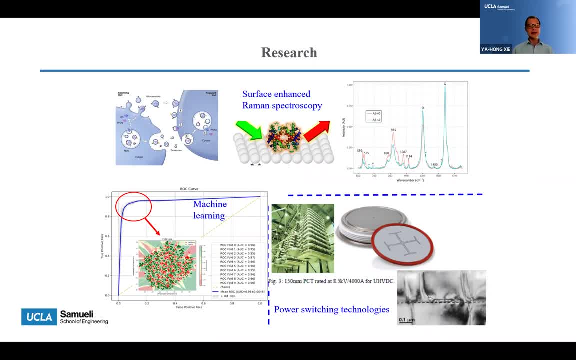 You'll try to watch the shape change. And also if you excite the material with light or electrical stimulation, then that will more likely to fall in the category of electronic material. So my research, starting from 100% electrical engineering, sort of the first step in my research. 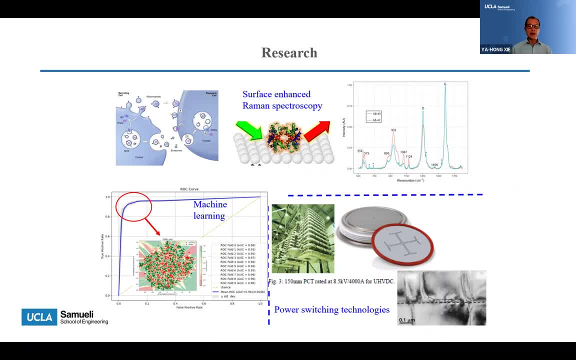 is sort of electronic material, let's call it So. we structure materials for exploiting certain electronic response. Till today, my biosensing portion of my research is really about also about the stimulation of the material using optical signal, And we try to extract information. 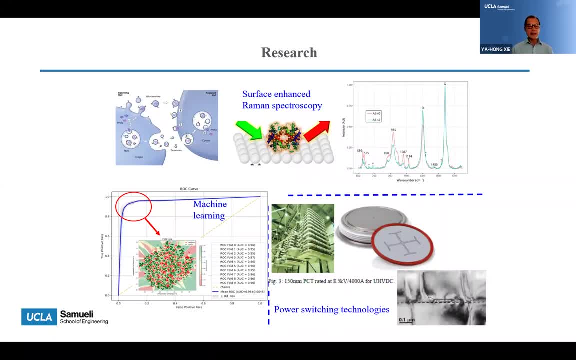 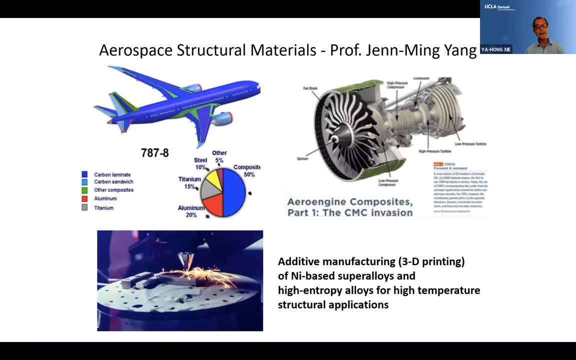 about biomaterials. So that's it. Next slide, please. I guess that's all. That's all my part. Okay, welcome again to UCLA. Great thanks very much, Johan. You know, I'm glad I passed you after all in that class. 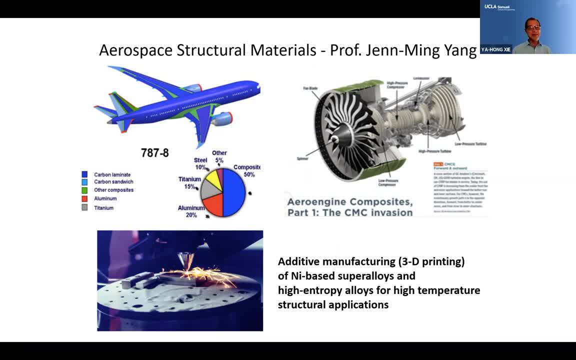 That's the thing I feel lucky. If I do it again, I may not be able to pass Right. Okay, And so next is going to be Professor Jianbing Yang. Good morning and welcome to UCLA. My name is Jianbing Yang. 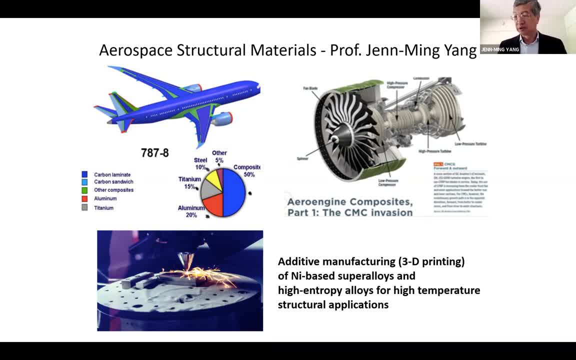 My research covers a wide spectrum of lightweight structural materials for aerospace applications. A few examples, including carbon fiber reinforced composites For airframe. as you can see here, Boeing 787 and Airbus A350,. they are using carbon fiber reinforced composite as the major airframe material. 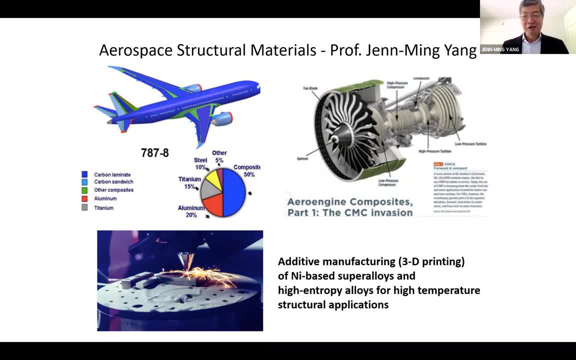 instead of using the aluminum alloys. okay, But, as you probably will know that, if you look at Boeing 787 and Airbus A350, they use a different type of carbon fibers, they use a different manufacturing approach, they use a different design methodologies. okay. 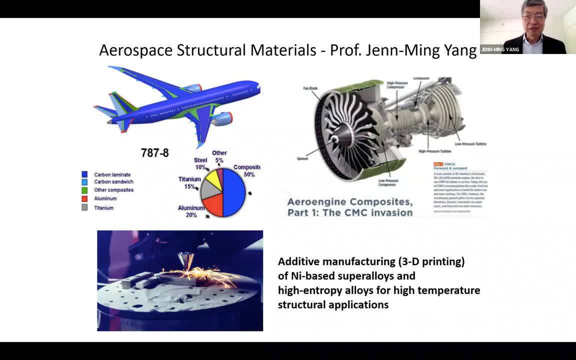 So there's lots of challenges of how do we assemble these very intricate structures for aerospace application with very good damage tolerance and durability, okay. So the second example I'd like to show you is to look at the aircraft turbine engines. As you have probably read the news, 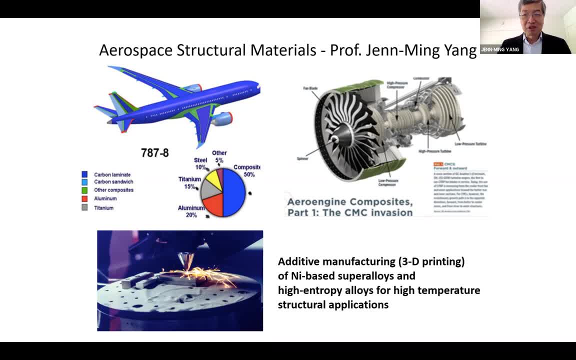 that back in the late February United Airlines Boeing 777-200 had an engine fire in midair. okay, So the preliminary investigation from FAA indicated that if you look at the front end of the engine, the fan blade for that Pratt & Whitney engine. 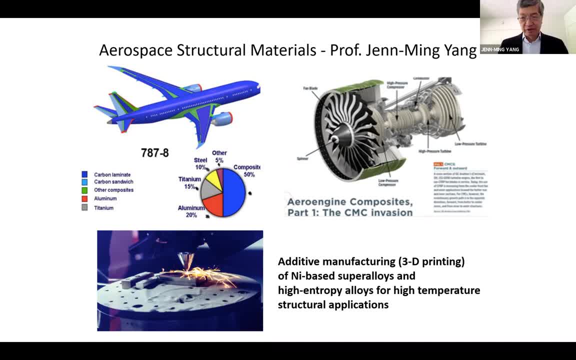 is made out of traditional titanium alloys, So metallic material are very prone to fatigue induced failure. So you need to do a very regular inspection to ensure that there is no cracking. as Professor Tan just mentioned about the material failure And some of the newer generation of engine, 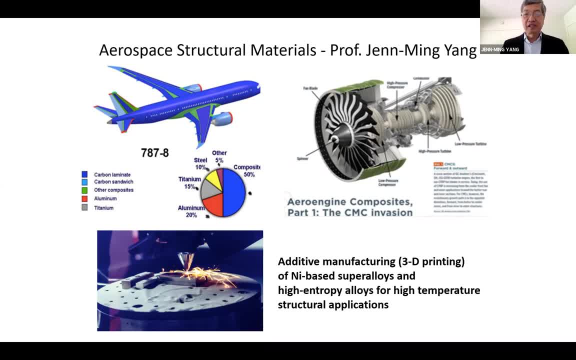 in fact, that this fan blade is no longer a titanium alloy. It has been replaced by carbon fiber epoxy to reduce the weight, to improve the life and also to improve the fuel efficiencies. Looking back at the engine, there are many, many high-tech engines. 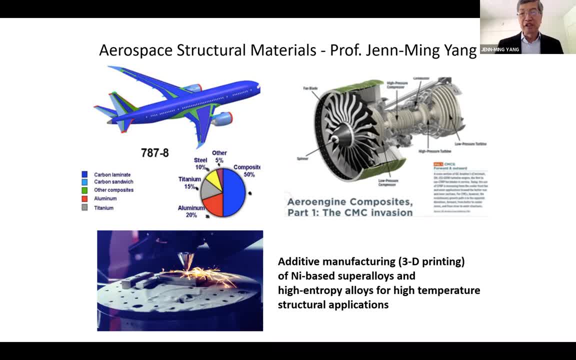 high-temperature structural materials, which are all based upon nickel-based alloys, which are quite heavy, okay. So various engine companies are developing new generation of turbine blade materials- okay, Based upon ceramic matrix composites like fiber reinforced ceramics- okay. 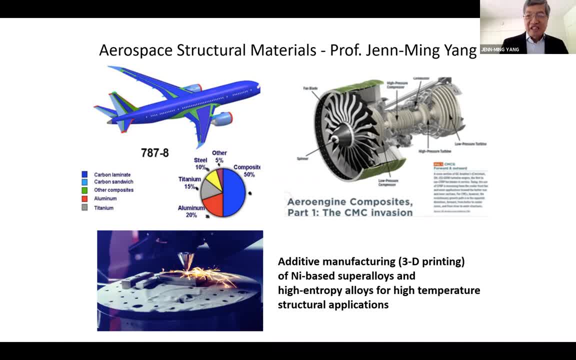 To reduce the weight, to reduce the needs for aircraft coolings and so on. So this is again. you will see that for the new generations of engines, new materials are being implemented into the aircraft turbine engines. okay, In the third example. 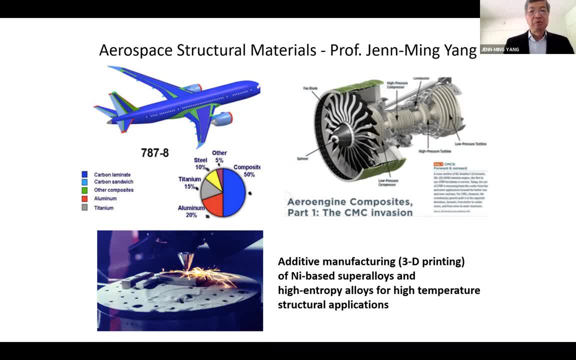 in which Professor Wang has just mentioned. okay, We did a lot of work on additive manufacturing, or 3D printing of nickel-based super alloys for, you know, rocket engine applications. We're also working on high entropy alloys for these hypersonic aircraft applications. okay, 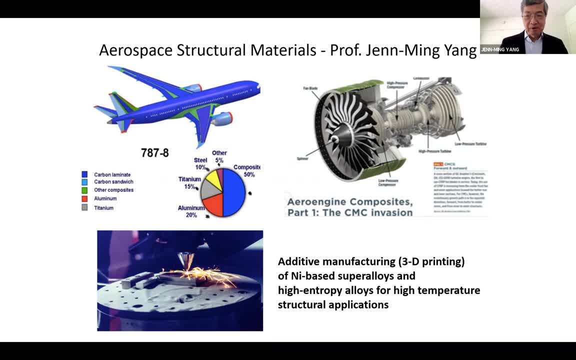 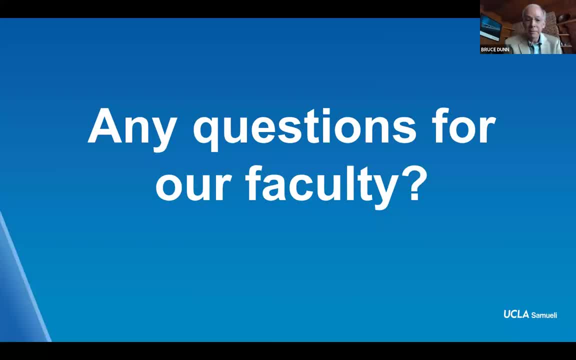 And we welcome the undergraduate students to join our laboratory to work on these projects, Thank you. So there's questions, but let me just mention one thing For those of you who are deciding about whether to come here for your undergraduate education: we are what you're seeing. 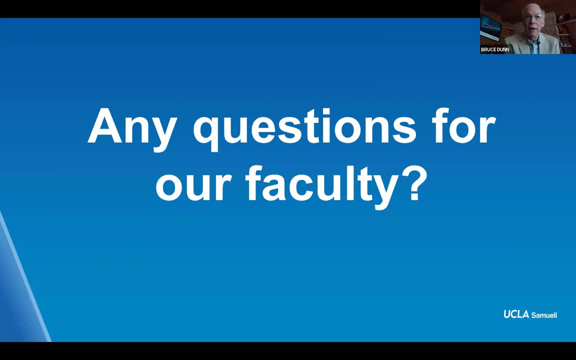 are very sophisticated applications. If you didn't understand all of it, don't worry about it. If you didn't understand part of it, don't worry about it. That's the kind of stuff you learn. The main thing is that our students learn this over the time. 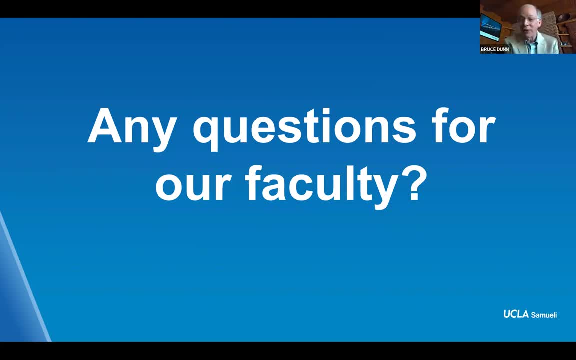 so that, even though you might go, I can't possibly imagine learning this. No, that's not the case. You will really. you'll be brought into this And you'll have the background and the full understanding. So that's the, that's my pep talk. 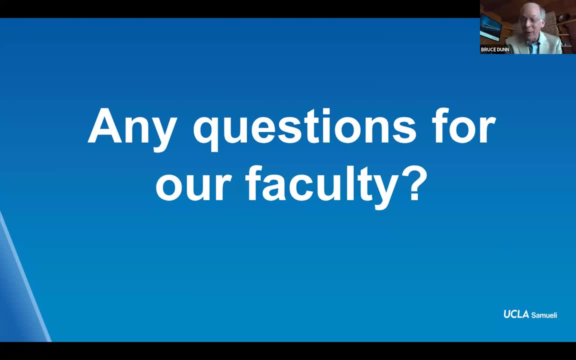 So I'll let you know that. don't worry, We, this is what we do. We educate students With that. any questions for us? You can use the chat or raise hands. either way. You can also unmute yourself and ask. 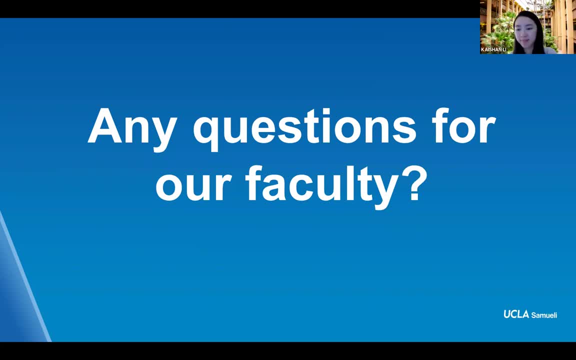 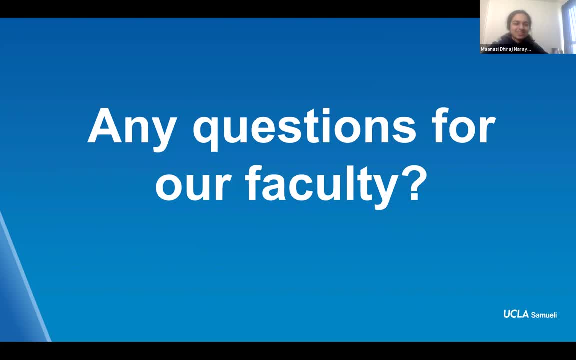 I was wondering, since materials science is such a rich and broad field, as you mentioned, And even today I learned- even even today I learned new applications that I didn't realize- How does the undergraduate education at UCLA allow us to explore the different applications? 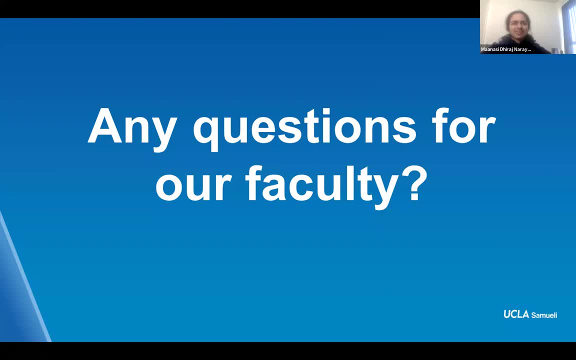 before we consider the prospect of joining one of these labs or even considering the research in these labs. That's a great question. So we teach fundamentals So that you understand fundamental properties: strength, electrical properties, optical properties. That's what we teach, And the best way to teach it is through examples. 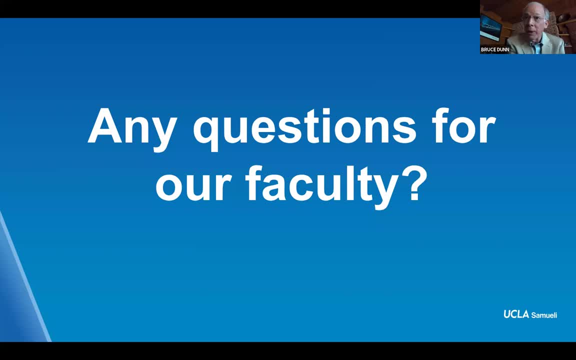 And so this is why research is so important, because the examples we bring into the classroom are of the latest research, And so this way, you are introduced to literally state-of-the-art, because those wind up being the best way to show how different materials behave. 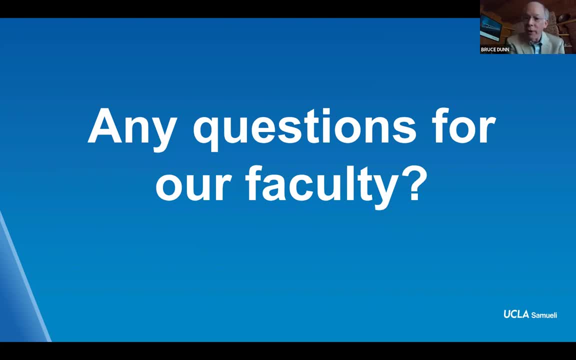 That's really about it. Now, as for joining laboratories, that's really something I think that the MRS student group- when you talk with them, they'll probably have some really good tips about that. Basically, when our offices were open, students would just walk into our offices. 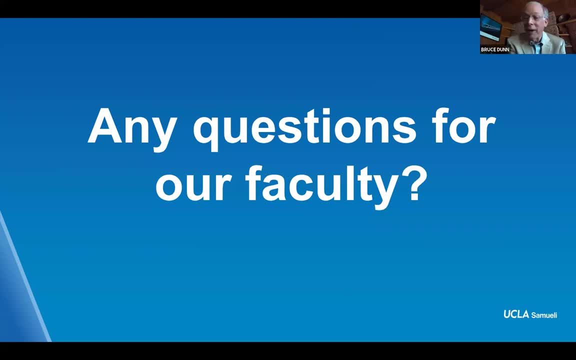 and say: what kind of research do you do And is there a position for me? And I'd say more than half the time the answer is yeah, we can find something for you to do. So I don't know if my colleagues join in, but it may sound a little haphazard, but we're a small. 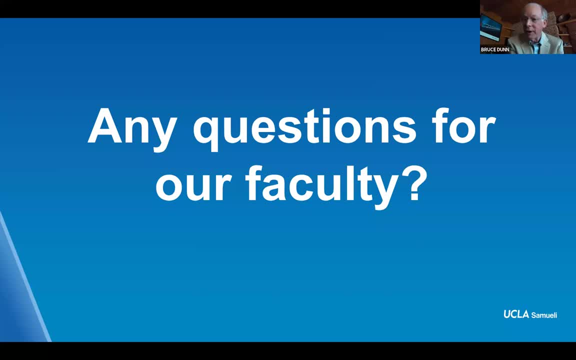 department- And that's one of the advantages of the small department- is that the faculty are always accessible. We got a few questions in the chat. Kyle asked there are a lot of graduate and undergraduate students compared to faculty. How easy is it to get to know faculty outside those quarterly meetings? 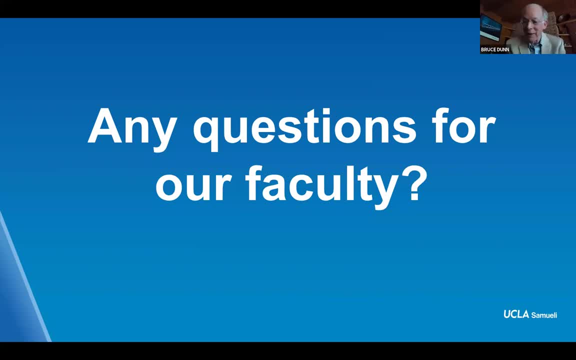 Oh, that's probably a best answered by the MRS students or our alumni. To know us is to love us, you know, Although maybe not everybody agrees with that. I don't do one of the students like to answer that. Yeah, I guess it's not really the time for student answers, but I'll jump in. 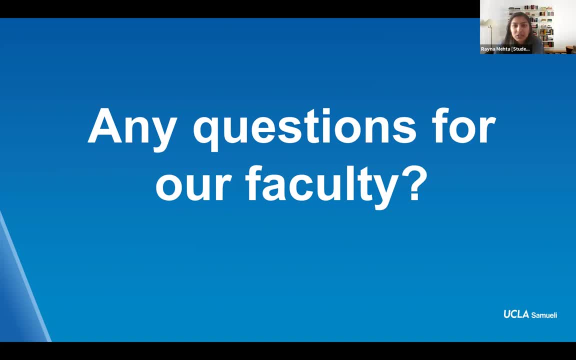 I think it's really easy to get to know the faculty. As Professor Dunn mentioned, it's a really small major. So even if you don't say anything in class, somehow your professor automatically knows your name And it's really easy to kind of get in touch with them and get to know them. And I think, like every 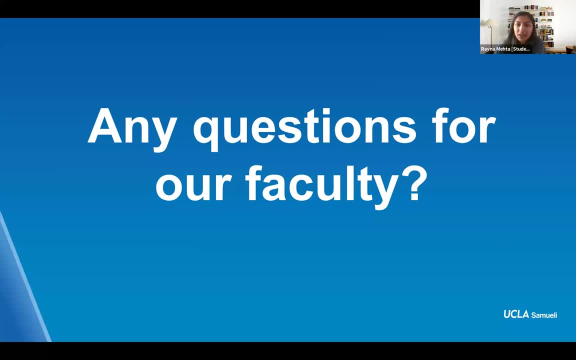 time I've emailed like a professor and said, hey, can I meet up and ask you about something? They've always been very willing to do so. So I think it's really easy to get to know faculty outside of just having your one faculty meeting per year, which you can also have more of if you want. 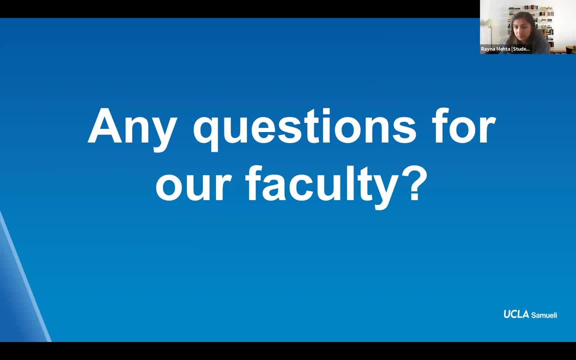 Okay, other questions: How does an undergraduate student go about finding research opportunities? I think I'm going to leave that for the MRS people. I will leave that for the next session, because I think that they're the ones that are in our labs. 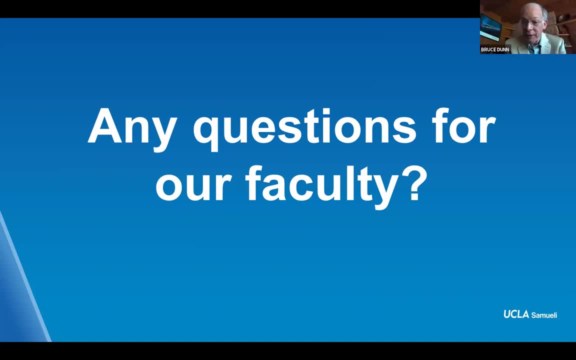 As I think I mentioned from my standpoint, I get contacted or people walk in the office and that's basically it. So it's really very individual on an individual basis, the way that I would look at it. Then one more question before we move into the next session. Someone asked: is teaching more theoretical or particle? 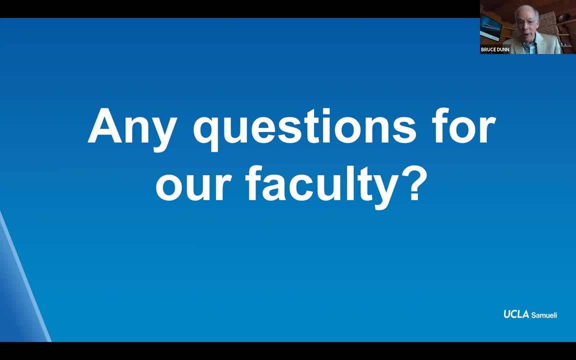 It's mixed. Some classes are more theoretical and others are really very much towards applications, And so that's the more practical side of things. We have laboratories, laboratory classes, which are designed to give you hands on experience in a variety of different areas that have to do with preparing materials and characterizing materials and different types of 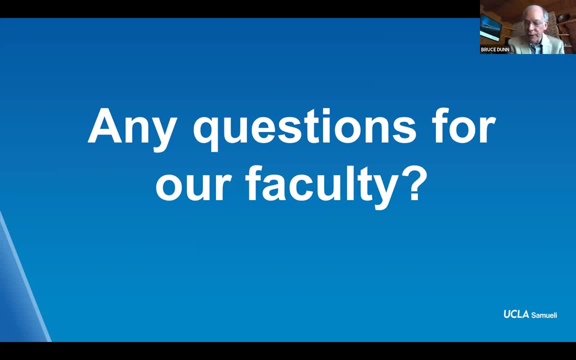 skills we hope are developed in those. So it's designed to be a mix. I should also add that, by various measures, we're considered like, without question, close in the top 10 of all the public schools to be in as for our undergraduate program. So so I think we do a good job of this. 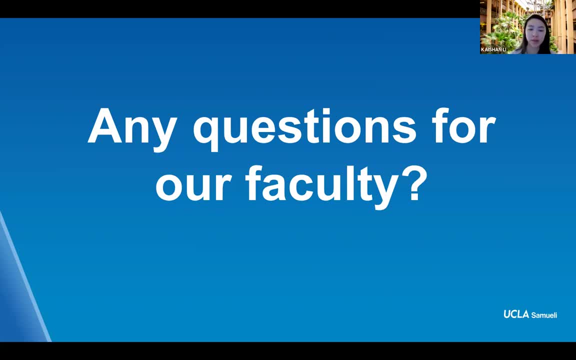 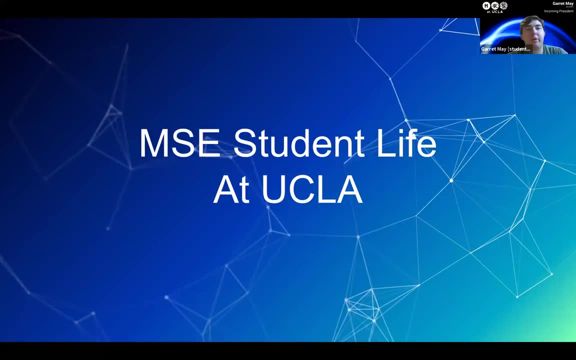 We have to move on, but there will be more opportunities for you to ask questions. So next up we will have our MRS students. Hi everyone, my name is Garrett- I use he, him pronouns- and I'm a current UCLA MathSci student at UCLA. Hi everyone, my name is Garrett, I use he him pronouns and I'm a current UCLA MathSci student at UCLA MathSci. Hi everyone, my name is Garrett, I use he him pronouns and I'm a current UCLA MathSci student at UCLA. Hi everyone, my name is Garrett- I use he him pronouns and I'm a current UCLA MathSci student at UCLA. Hi everyone, my name is Garrett- I use he him pronouns, and I'm a current UCLA MathSci student at UCLA.